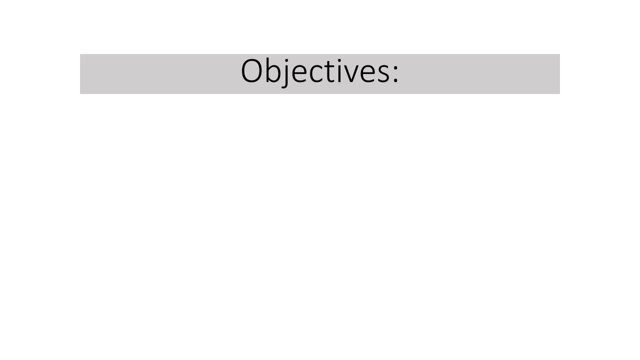 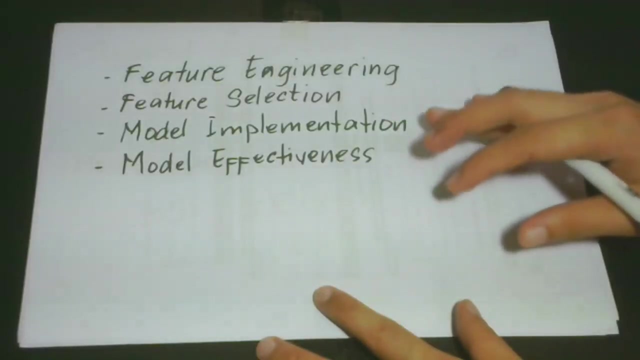 At the end of the lesson, you are expected to identify the supervised machine learning evaluation metrics for regression, compare one metric from the others and appreciate the significance of evaluation metrics in machine learning. As a data scientist, you know exactly that we are actually doing a lot of things in our data science project, So among this we have the. 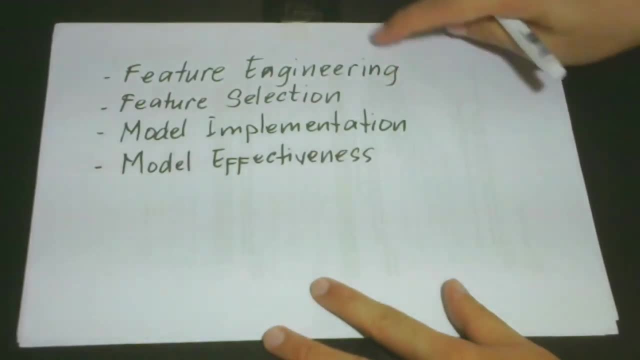 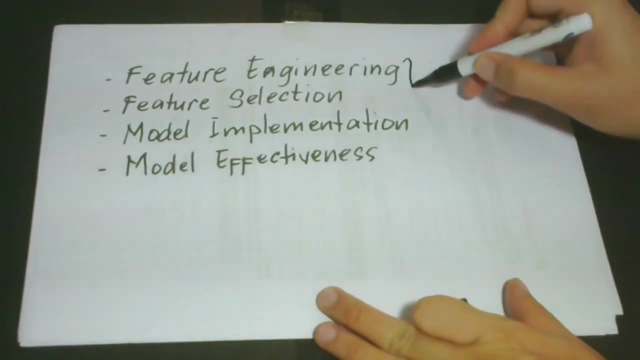 feature engineering. We do have the feature selection, which is also a part of our feature engineering, And after that we build our model and then we do the model implementation. The next challenge for us to do is that what would be our next thing after we are done with all of these? 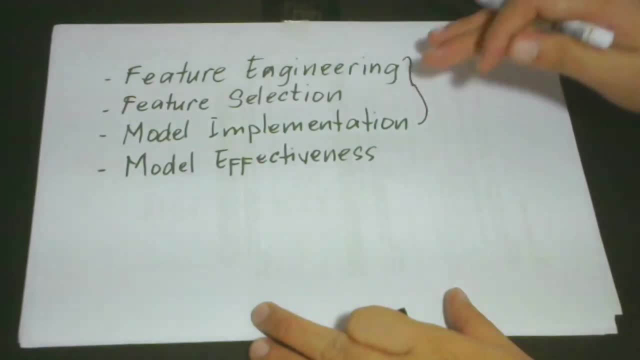 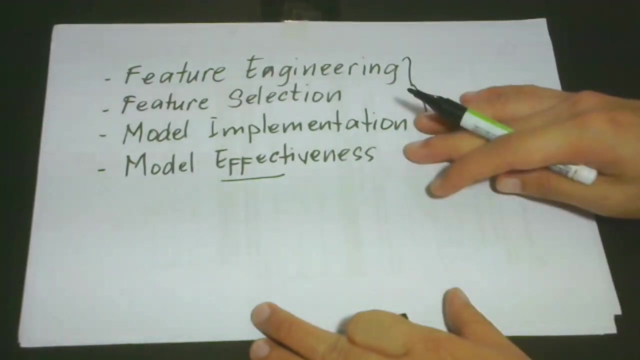 things. So when we do have a model which is already implemented, the next thing is we need to test and identify whether or not a certain model is effective. So here comes the comparisons and differences of the different results of the accuracy of our model. So now the question is this: how are we going to test the accuracy? 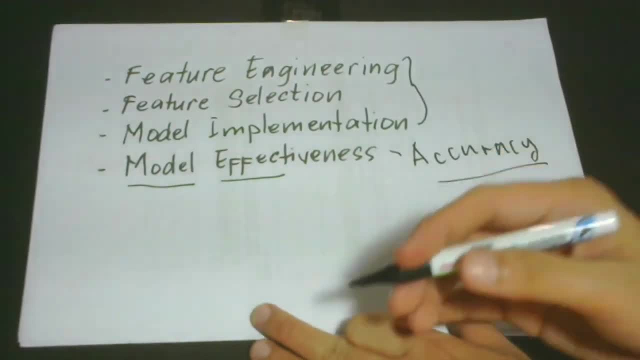 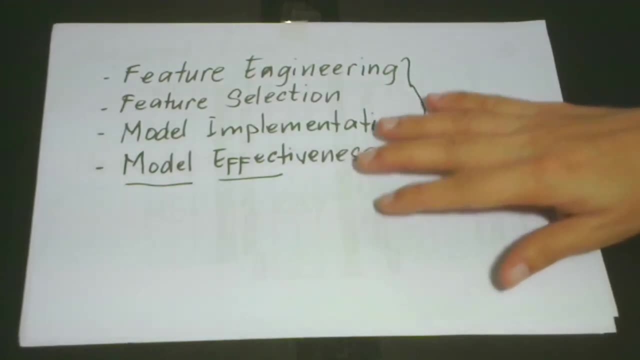 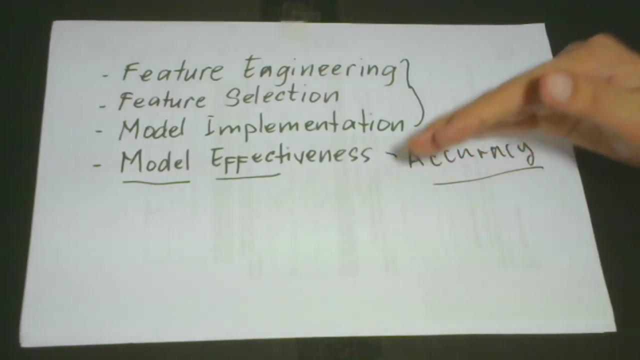 or the effectiveness of our model, And this is what we're going to have for this lesson. So before we continue, please don't forget to hit that subscribe button down there to enjoy our data science free courses like Mastering Machine Learning, Algorithm, Deep Learning, Mathematics, the different data science algorithms and many. 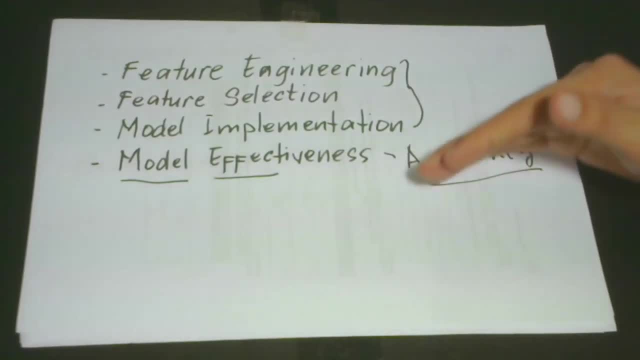 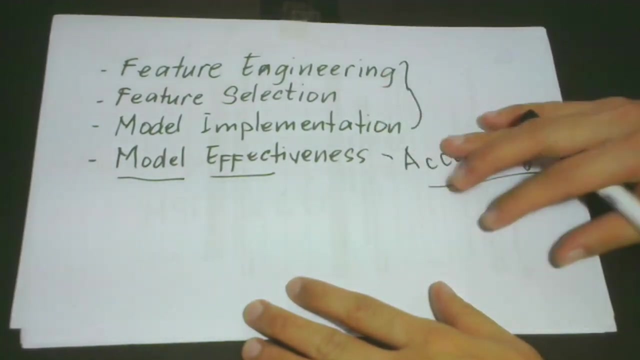 more. Please don't forget to hit the notification bell to be able to be updated of what's going on in our channel. Give this video a thumbs up and share this with your friends. So we're going to have, one by one, of the different evaluation metrics of our regression. 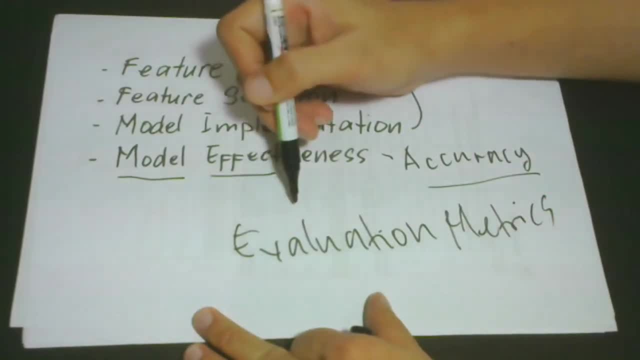 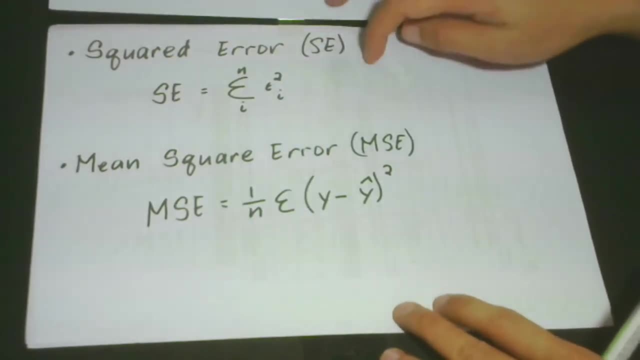 Let me write here. So we are going to have the evaluation metrics of a regression. Let's first have the squared error. So what is this squared error all about? So basically, what we do here is that we square the actual value minus the predicted value And then we do the summation of all of the. 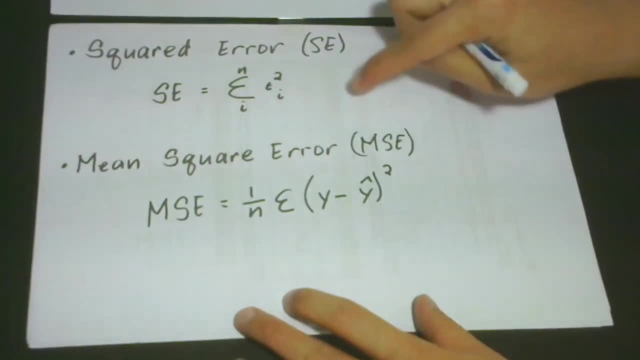 outputs. So maybe you would like to ask me what's the good thing of using the squared error in our regression model? So the good thing of using the squared error is that we would be able to evaluate the accuracy of our regression model. One of the advantages of using the squared error is: 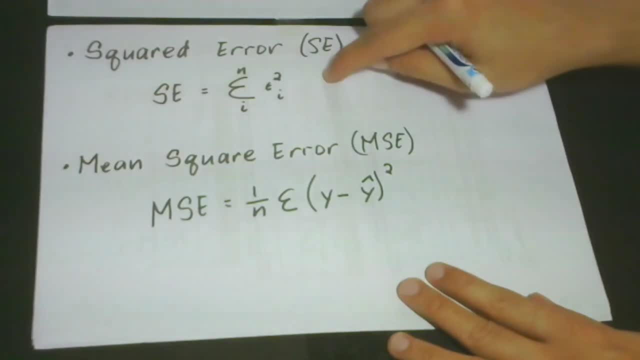 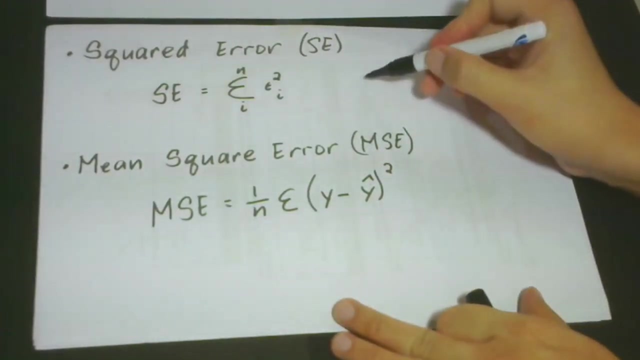 that we would be able to identify how dispersed the values of the errors, at least on average. And when we do the squaring of the error, we are actually penalizing the observations which are too far from the fitted line. So, for example, when we have this line and when we have a lot of points, 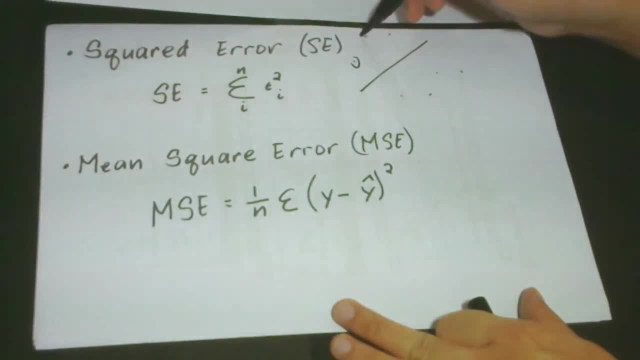 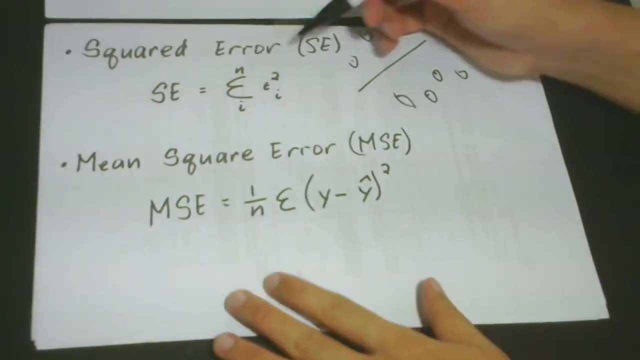 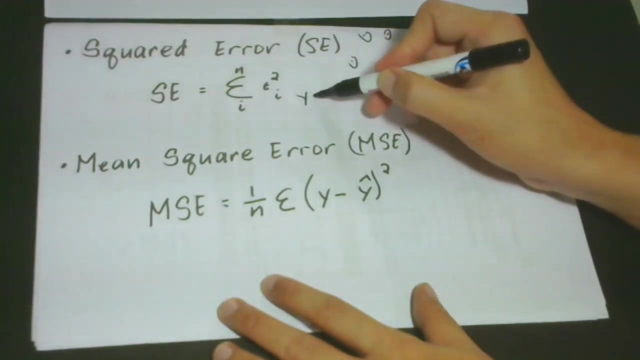 too far away from the line we would be able to find the error. So we would be able to find the error in our line. Then we are penalizing these ones by squaring the differences from the predicted line. So again, the error here is we get the difference of the actual value and the predicted value. 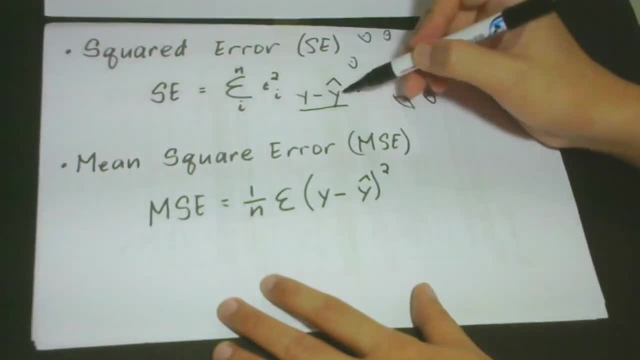 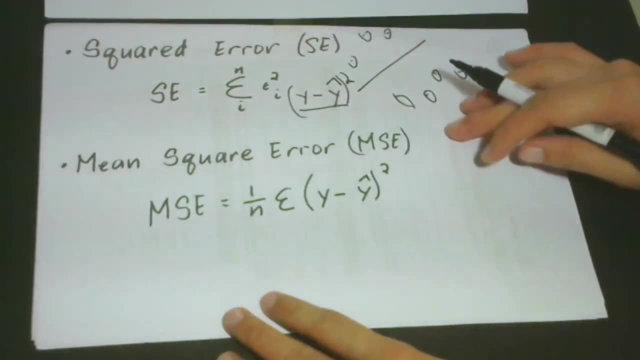 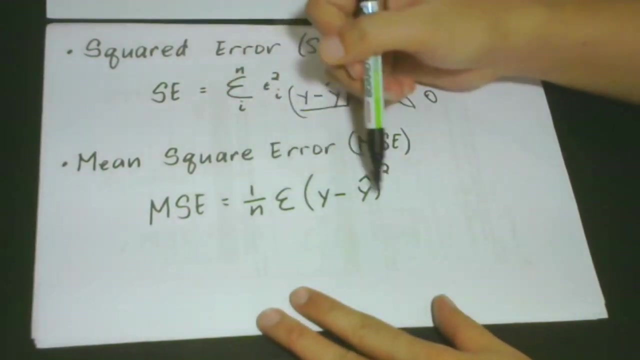 So this is the formula of getting our error. Of course, we square this and this one is our squared error. Now let's go to our mean square error or MSE. How do we get this one? So this is the formula of getting the mean. 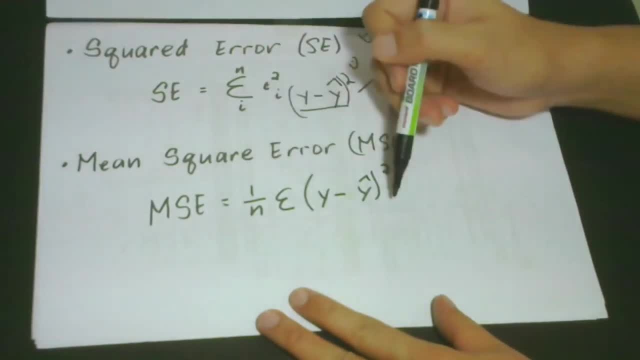 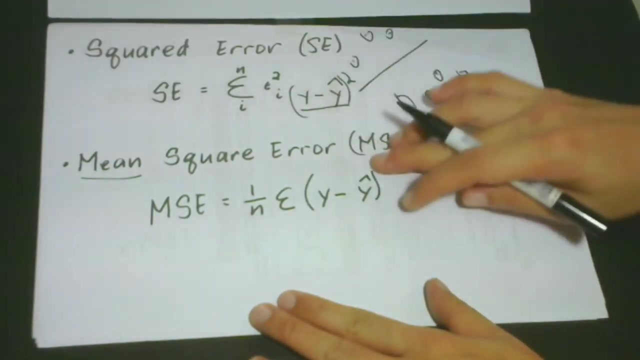 square error, And just by seeing the formula itself we could say that this is actually the squared error, but only that we divide that with the total number of observations. So that is why we call this one the mean In comparison to the squared error, which penalizes. 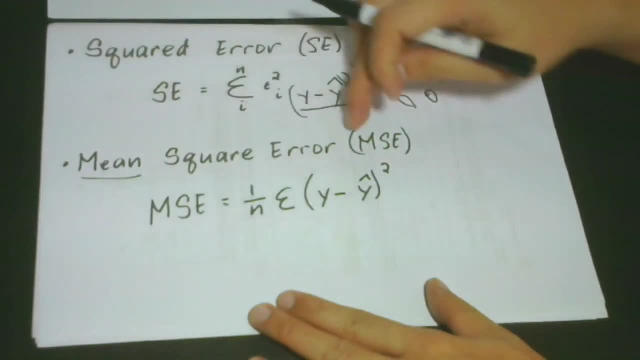 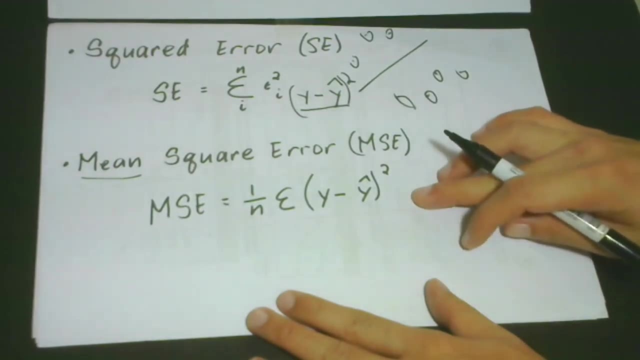 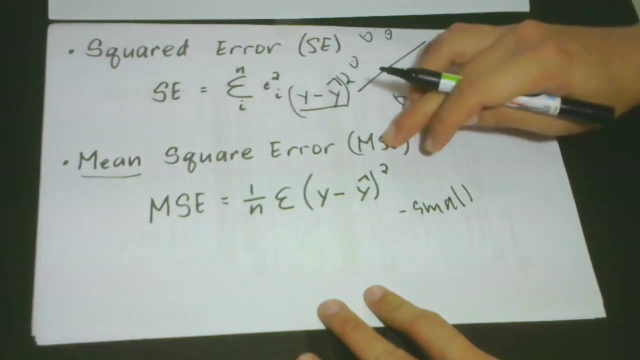 the larger ones. in the case of mean square error, not only it penalizes the larger points, it also penalizes even the smaller points in our dataset. This kind of metric, or evaluation metric, is more preferable than the squared error, because in the first place this is differentiable and this one can be optimized better. 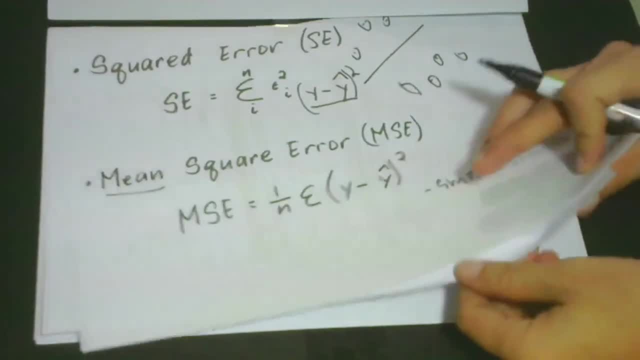 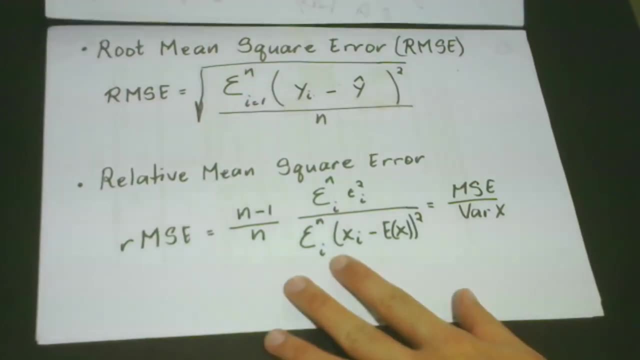 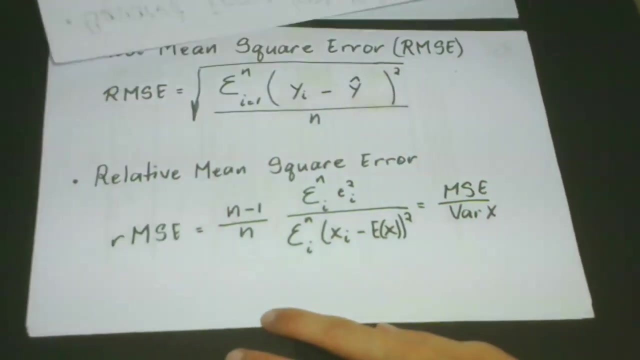 So now let's go to our next evaluation metric, which is the root mean square error, or RMSE. So what this one is all about. So root mean square error is actually our mean square error, but only that. the difference here, in this case, is that we get the root of the. 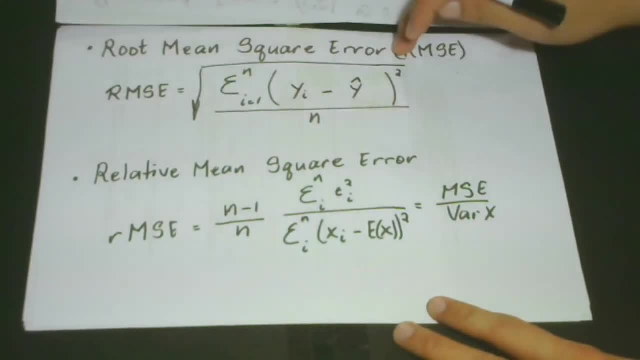 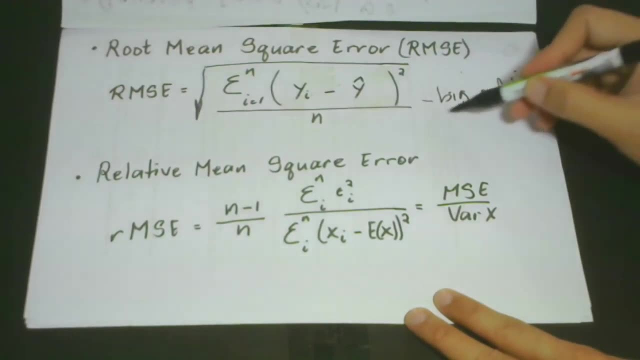 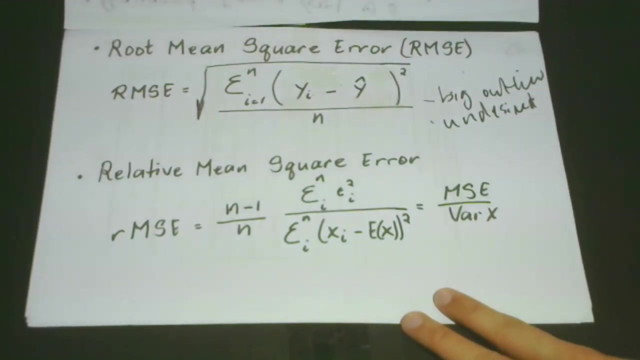 mean square error. So when do we use this one? So in cases when we have very big outliers and these outliers are very undesired, then we can use the root mean square error to test the effectiveness of our regression model, And then we have the relative mean square error. 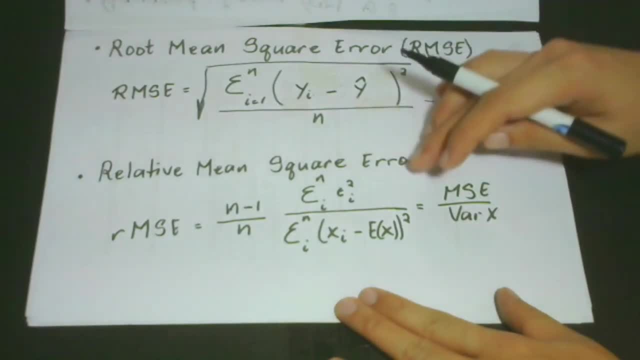 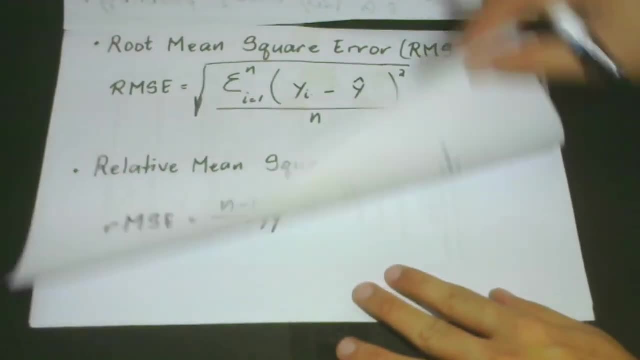 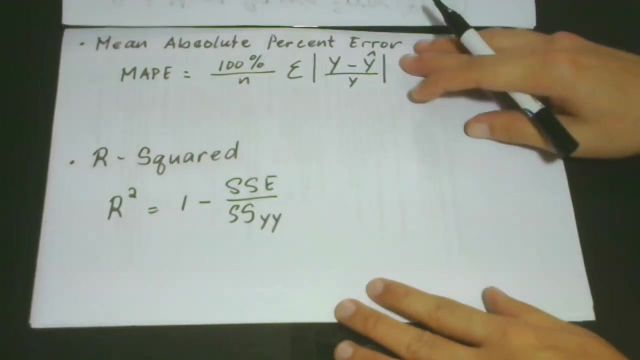 And what do we do in this case? It's very simple. This is actually the MSE of our model divided by the variance x. It's very simple. Now let's go to our next evaluation metric, and this metric is the mean absolute percent error. So what this one is all about. So we get the MAPI by first getting the summation of the root of the mean square error. So what this one is all about. So we get the MAPI by first getting the summation of the root of the mean square error. So what this one is all about. So we get. the MAPI by first getting the summation of the root of the mean square error. So what this one is all about. So let's tell them. to Pokémon, the volume is equal to one third of the value x times 1.. So when we look at, 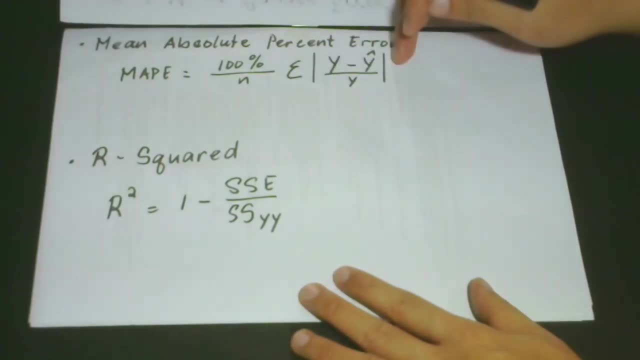 the representation of the multiple variable by nell. we previously had the, Yet the y minus y-hat divided by y, And take note that we get here the absolute value of the points And then we multiply that to 100% and divide that by the number of observations And this evaluation. 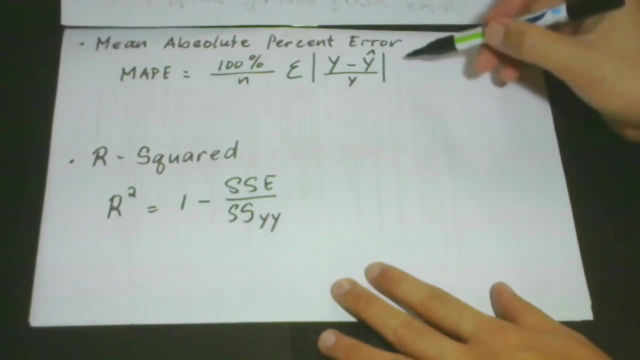 metric is very useful when we would like to check the forecast accuracy. So, forecast accuracy and with respect to forecast accuracy, the Eddie nine nil convolution, Awesome. By measure one, and that's equal to ye nine nil— that is compared to the total value. So medium is the variance of width. 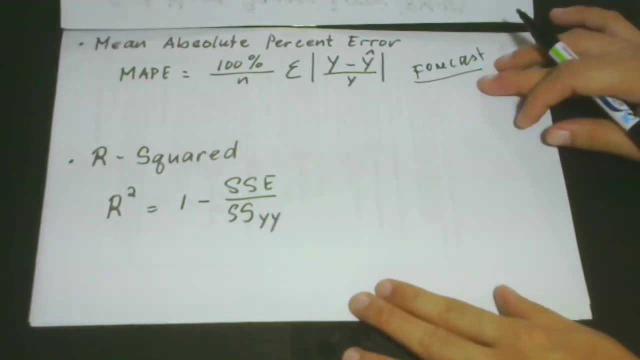 respect to forecast accuracy. this is always connected to time and speaking of time, we are comparing here series on different scales. but mean absolute present error has its own disadvantage, and this must be taken with extra care. and what is this disadvantage of our mean absolute present error, or mappe? this one tends to infinity and because this is so, sometimes it becomes undefined. 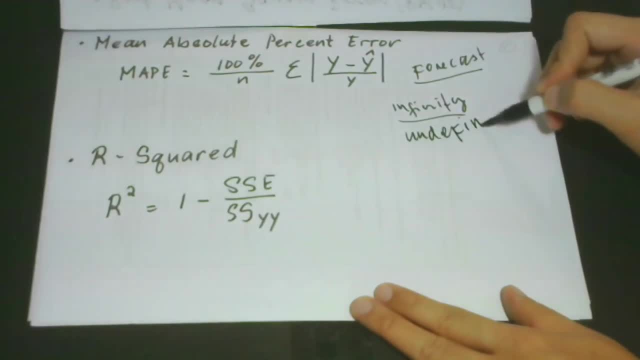 let me write this one undefined, and maybe you would like to ask me when would be the situation when it becomes undefined? so it becomes undefined if the value of the actual figure is zero or any observation in our data. so with that we have to be very much careful. 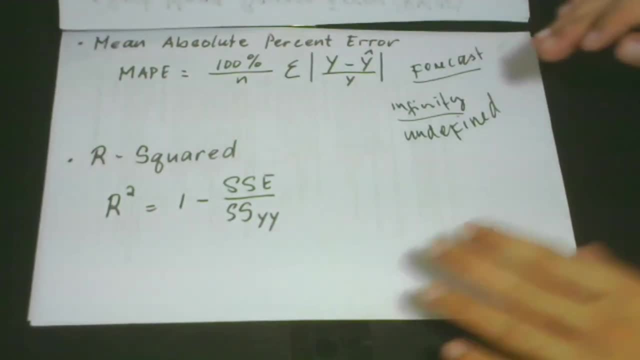 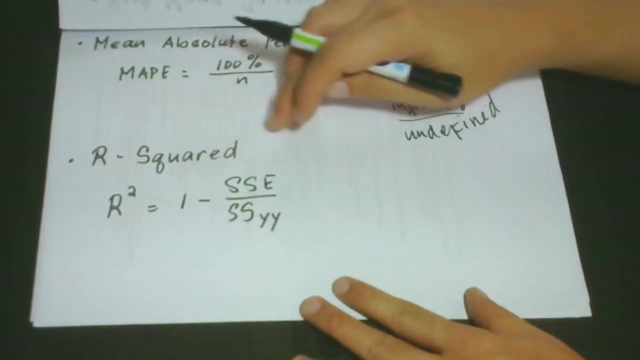 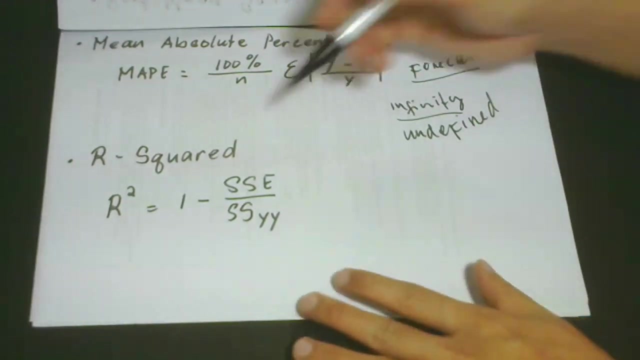 when we use mean absolute, present error, when we observe this kind of value in our data. okay, so now let's go to the r squared. what is r squared? and i believe that you are very much familiar with the r squared. so how do we get it? it's very simple. we get this one by deducting the quotient of sse. 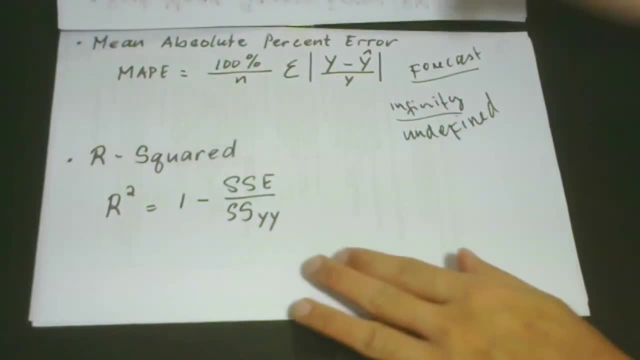 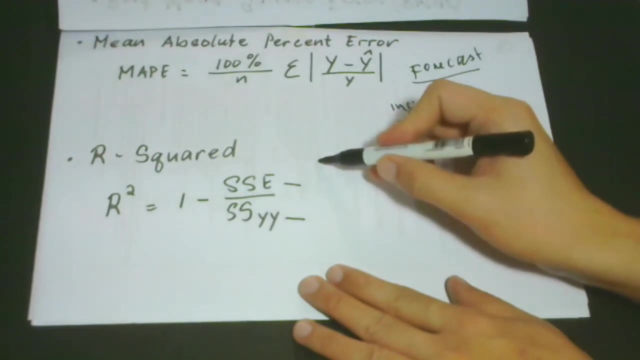 and ssyy to one, and maybe you would like to ask me what this one is and what about this one? so for you clarity, especially if you don't have any technical and statistical understanding of all of these things, let me give you this one. so this is the summation of the squared differences between the 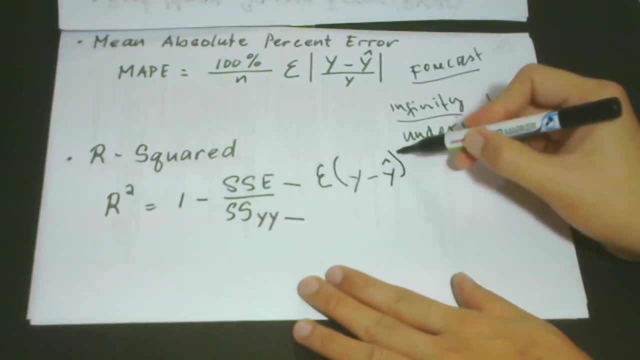 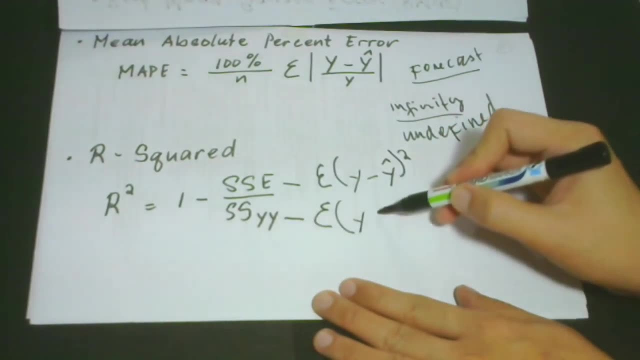 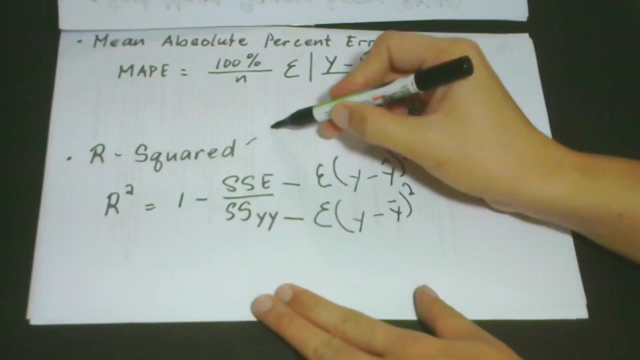 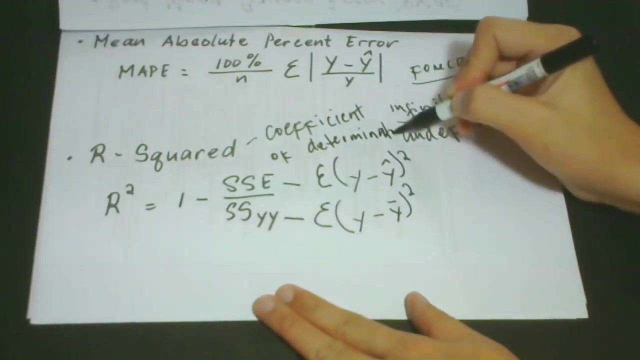 actual value and the predicted value. okay, and what about this one? so this is the summation of the actual value and the mean. so that's a difference, right and anyway. r squared is also called the coefficient of determination, let me write here. so, coefficient of determination, don't forget this one. so what's the usefulness of the r? 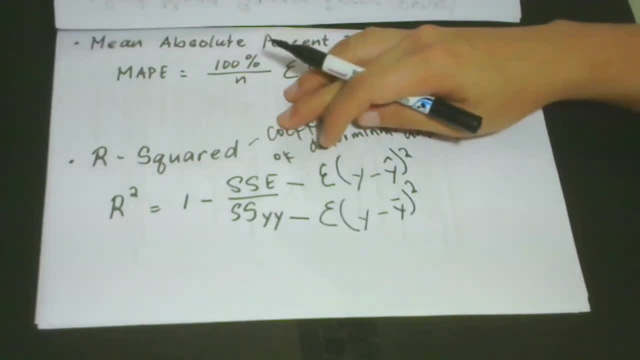 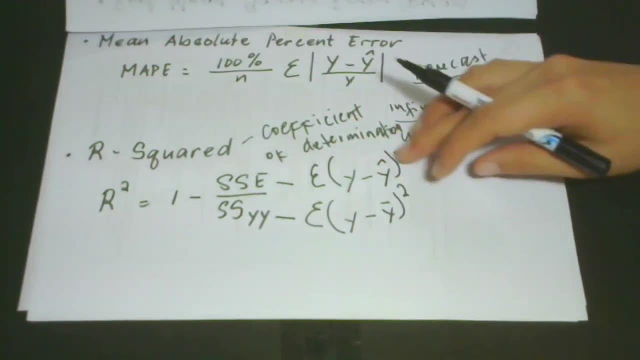 squared. so r squared is very useful if we would like to compare our current model with a constant baseline and with that it tells us how much our model is better. now let's go to our next evaluation metric, which is absolute, constant and constant femmes and runs through the equation value, and that is the result of the first step in our evaluation matrix, which is obviously average and positive. 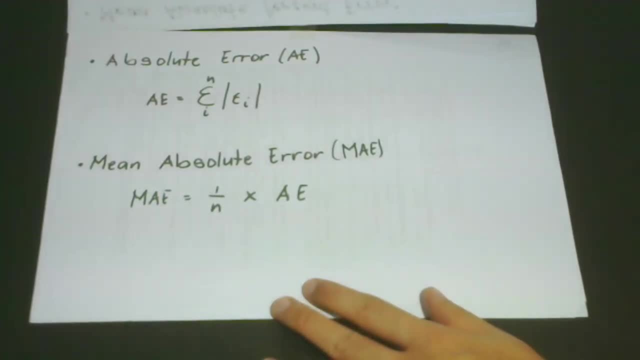 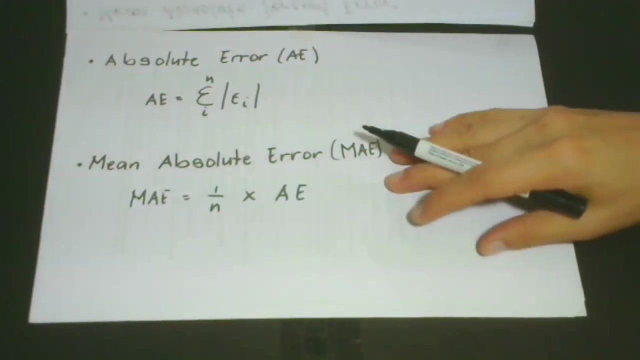 absolute error just from the name itself. we are taking here the absolute value of our error, and we know that our error is computed by deducting the predicted value from the actual value. okay, this is very simple. and our next one is actually a hybrid of absolute error, because in this case, 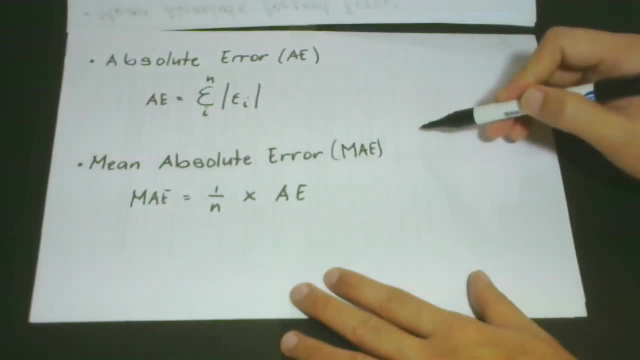 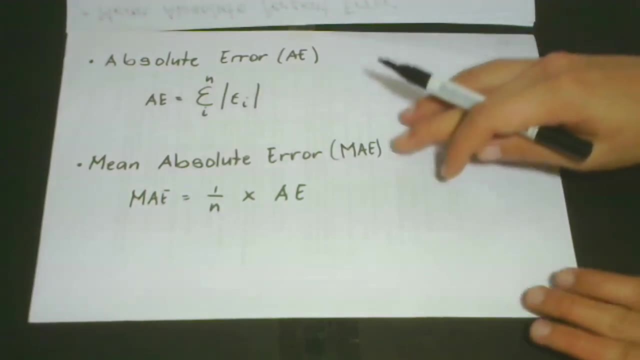 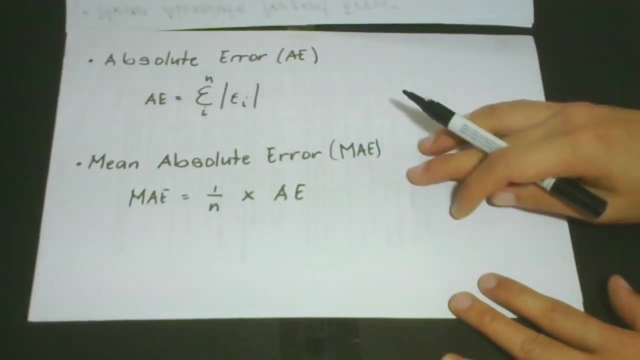 we call this one the mean absolute error, which is just: we divide the absolute error with the number of observations that we have. so mean absolute error is actually more robust to outliers and in comparison to the mean squared error it does not penalize the error in the most extreme scenario. 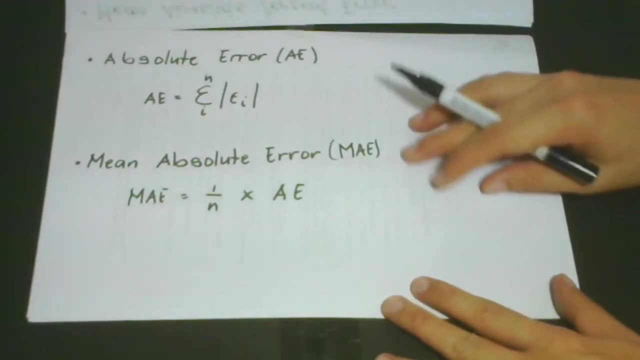 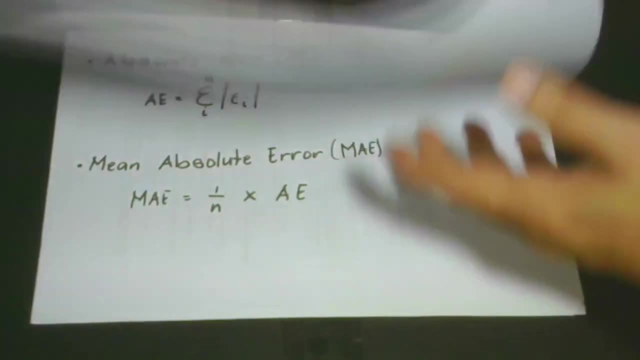 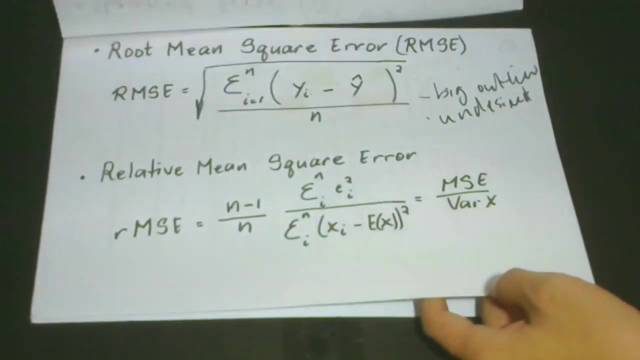 or value and in cases when we would like to pay attention to outliers mean absolute error is not applicable. so we have discussed the squared error or the se mean squared error or the mse. then we have the root mean square error or rmse. then we do have the relative. 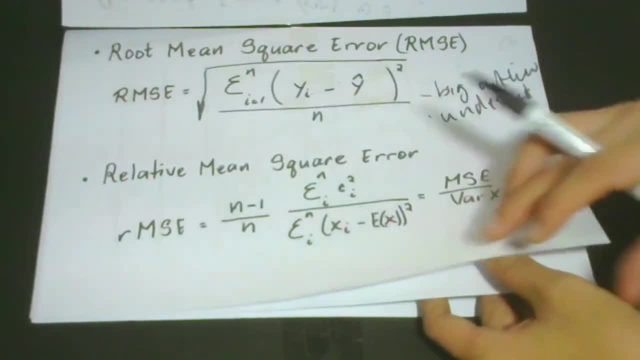 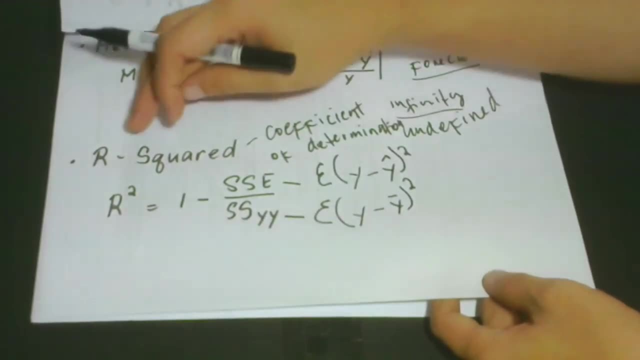 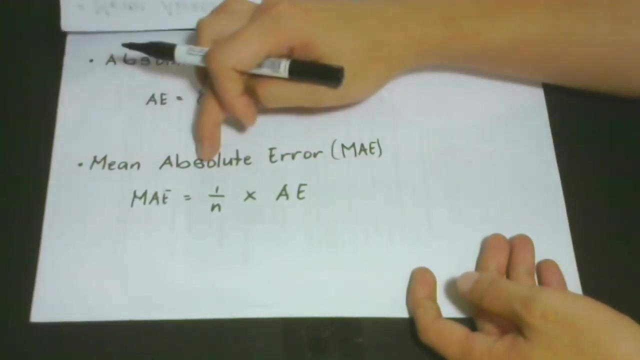 mean square error or rmse. don't forget the small r and the big r here. and we have the mean absolute present error. we also have the r squared. then we have absolute error or ae. then we have the mean absolute error or m or ma e. now the question is this: among all of these, 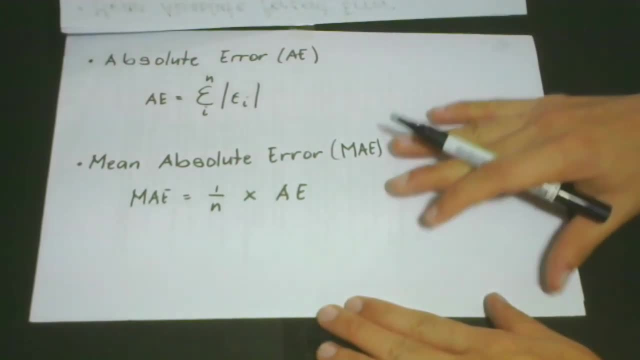 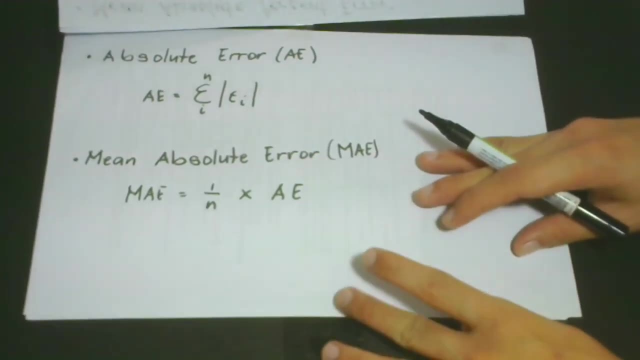 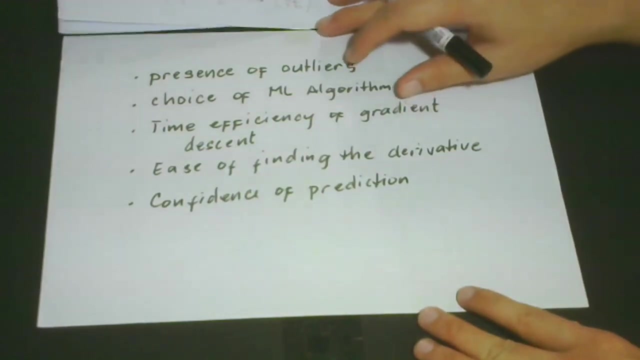 which ones are we going to use, or do we have the test to use for us to be able to choose from among them which one is the most applicable in a certain machine learning project? okay, that is actually a very good question, and here we have the different tests that we need to consider in choosing the. 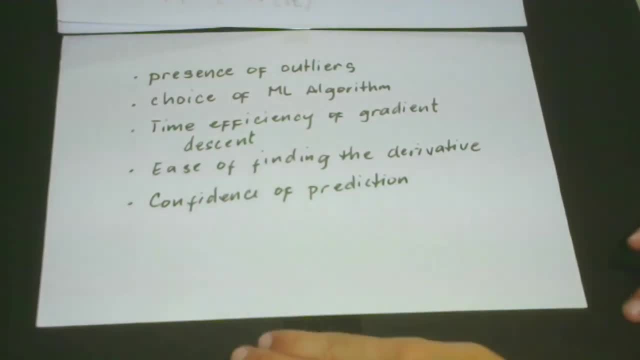 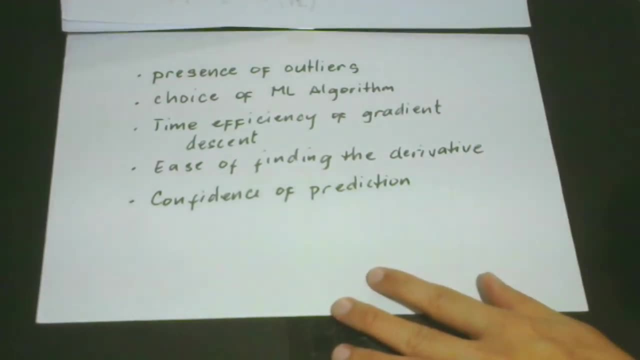 right evaluation metric in our data science project. i would like to point out that there is no most effective evaluation metric for all machine learning project because there are a lot of factors that we need to consider. So the factors are the presence of outliers. We have the choice. 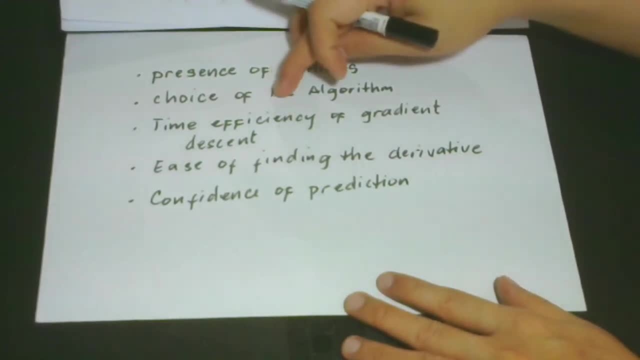 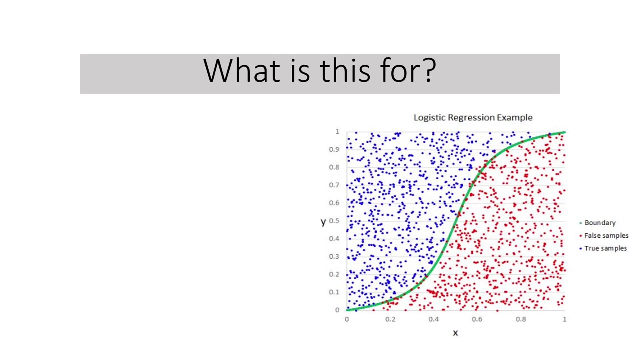 of machine learning algorithm, then the time efficiency and the gradient descent, the ease of finding the derivative, and we have the confidence of prediction. So you have to remember this one in choosing the right evaluation metric to use. What is this for? Why do we have to study this? 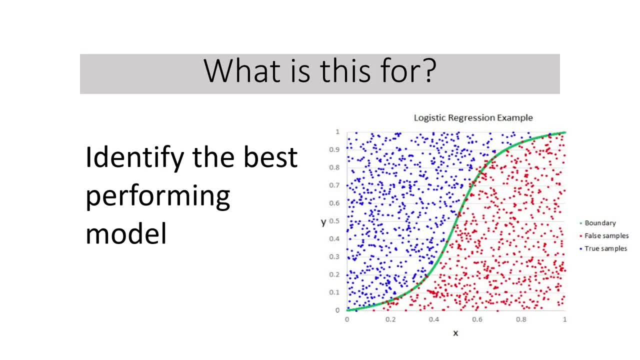 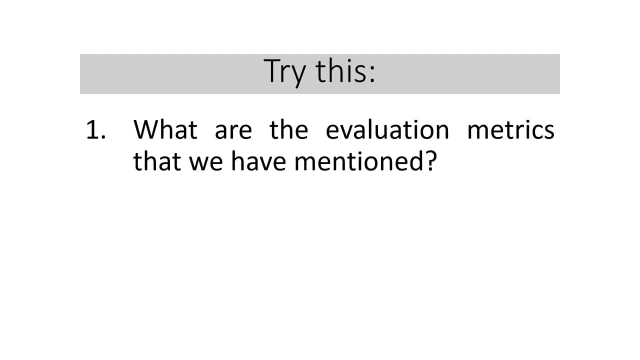 Knowing these evaluation metrics helps you identify which model to use that shows better accuracy and better predictive performance. This can save your time and money as well. After all, being said and done, let's try this. What are the evaluation metrics that we have mentioned? Can you explain the process of each one? Why are these evaluations? 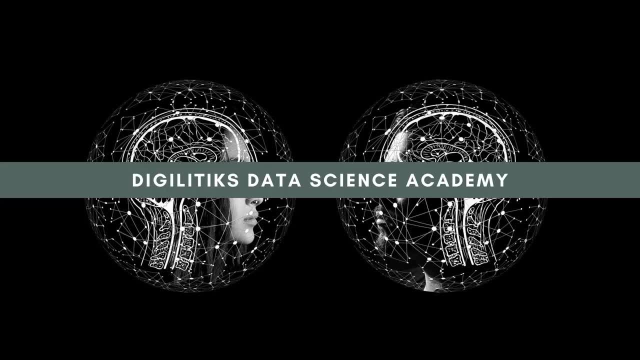 different. Why are they different? Why are they different? Why are they different? Why are metrics important in machine learning? Do you want to know more about this channel? Just click these cards. You can enjoy our data science courses for free, like Mastering Machine Learning. 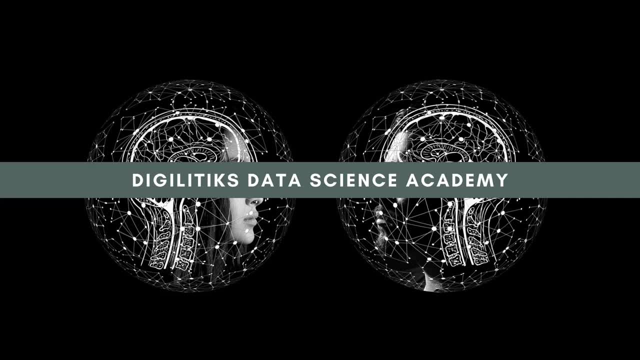 Algorithm, Deep Learning, Mathematics, the different data science algorithms and many more. Learn and upskill for free.